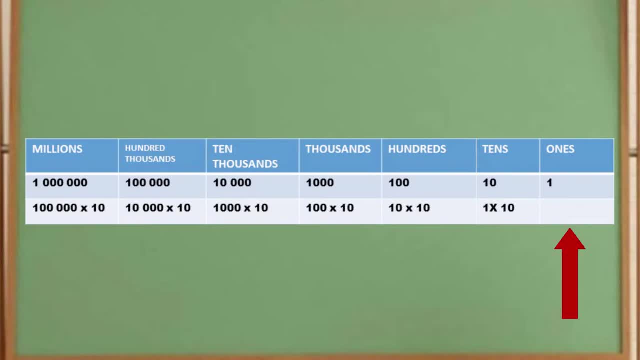 Look at the place value chart I have there. We begin with ones. Now, when we multiply that one by ten, we get ten. We move over to hundreds. When we multiply the ten by the value before, we get one hundred. We move over to thousands. 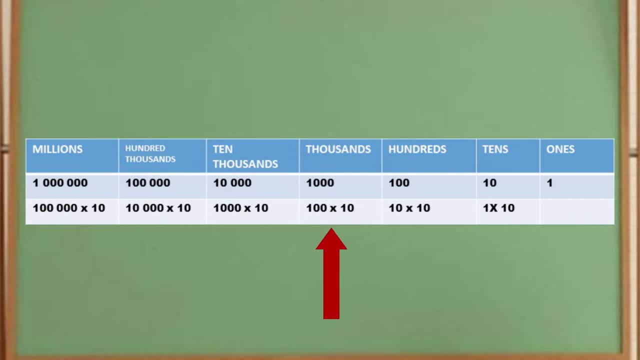 When we multiply the value before, which is one hundred by ten, we get ten thousand. When we multiply ten thousand by ten, we get one hundred thousand. When we multiply one hundred thousand by ten, we have a result. We have a result of one million. 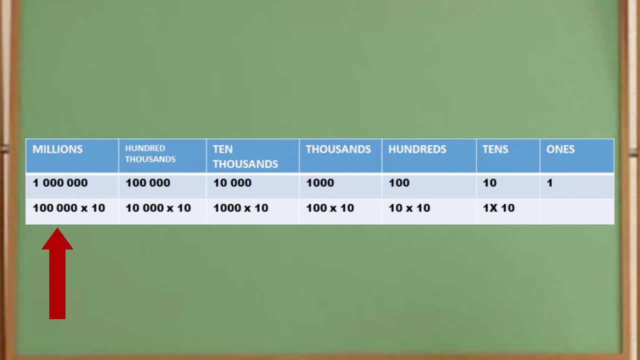 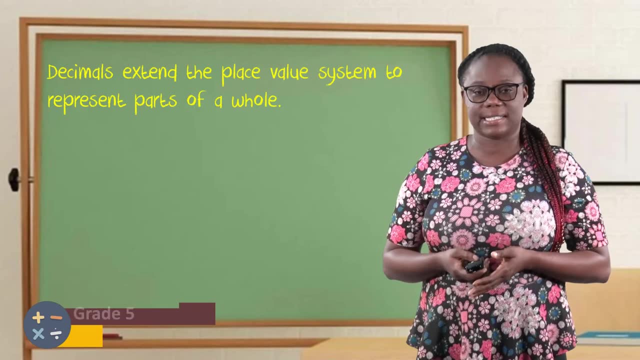 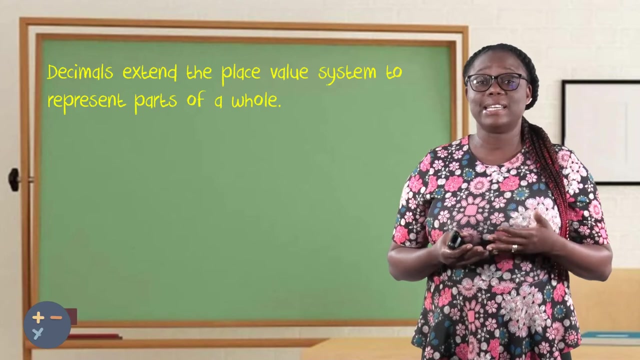 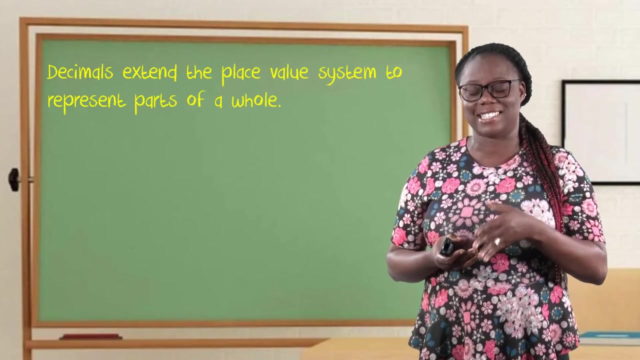 Boys and girls. do you see how the numbers are increasing as you move from right to left? Yes, Now for decimals, it's the opposite. Decimals extends the place value system to represent parts of a whole, just like fractions, It can be used to represent values in a whole. 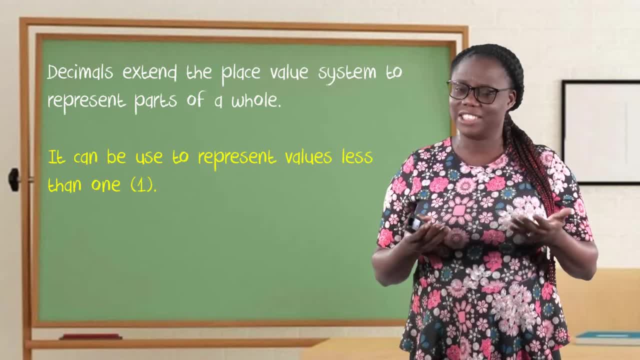 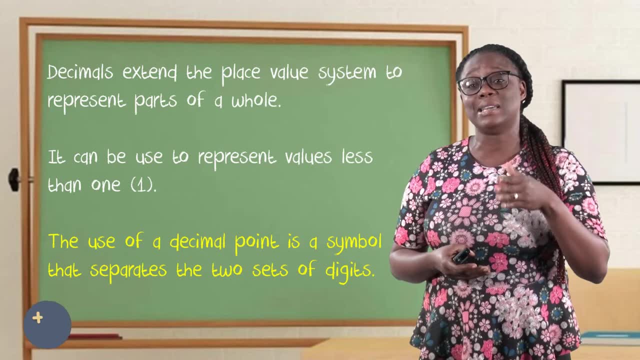 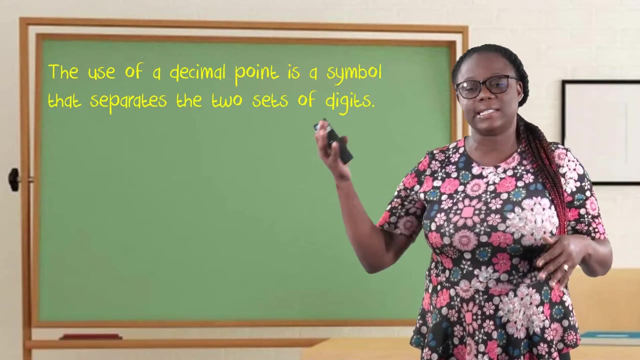 It can be used to represent values in a whole. It is less than one, just like fractions. The use of a decimal point, which is very important, is a symbol that separates the two sets of digits: The whole number and the decimal numbers. 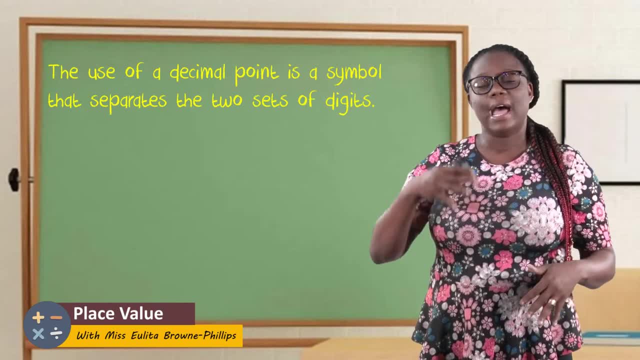 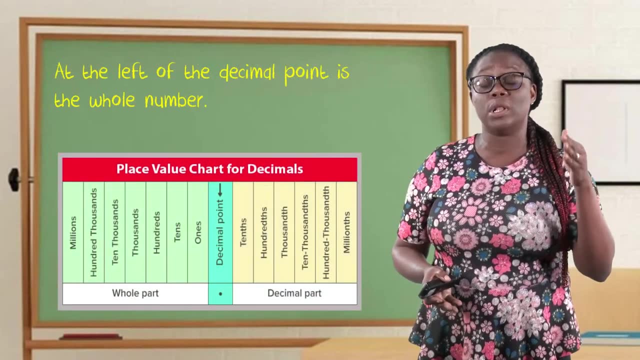 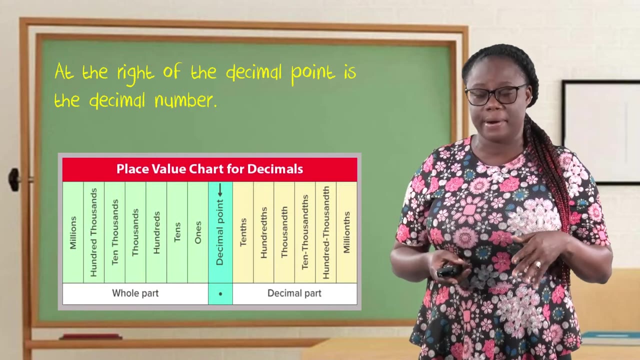 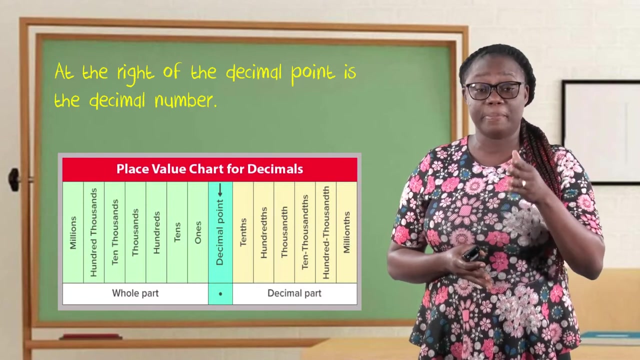 The part that is the whole number and the part that is the decimal. At the left of the decimal point is the whole number. At the right of the decimal point is the decimal number. look at the chart I have there. Do you see the decimal point in the middle separating the whole part from the decimal? 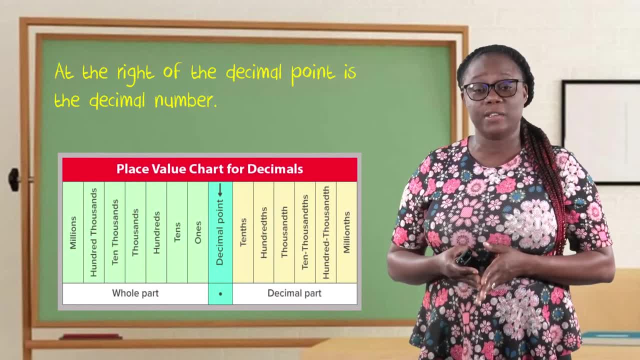 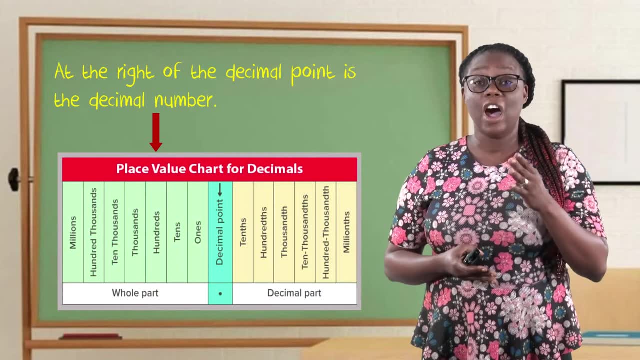 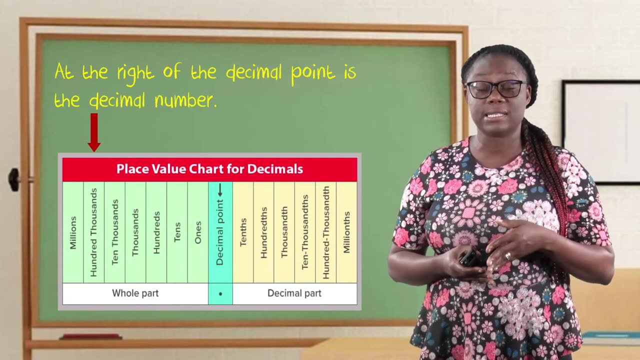 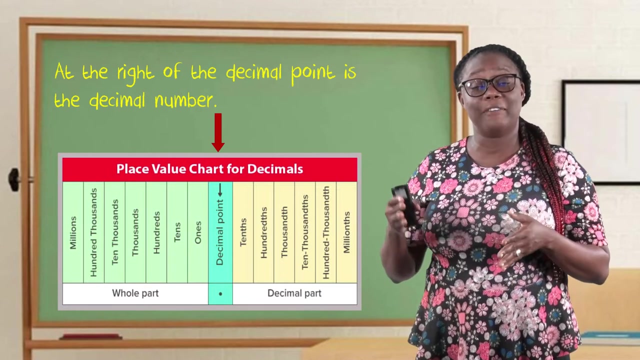 part. Let's look at the place values of the whole part. It starts with ones, tens, hundreds, thousands, ten thousands, hundred, thousands and millions. Let's go to the right of the decimal point. That's where you have the decimal part of the number. 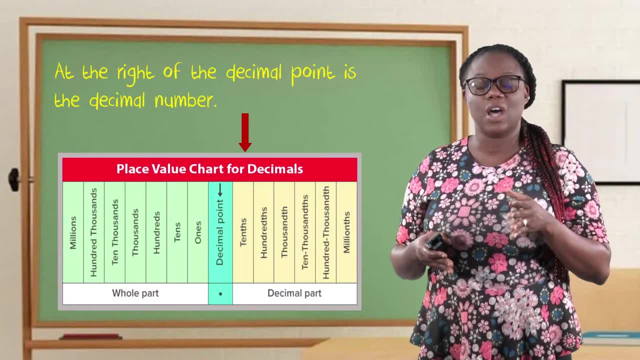 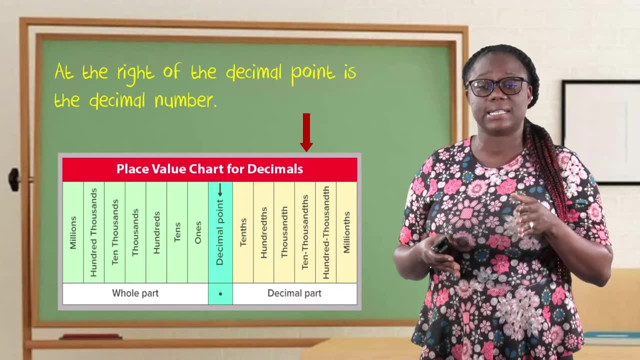 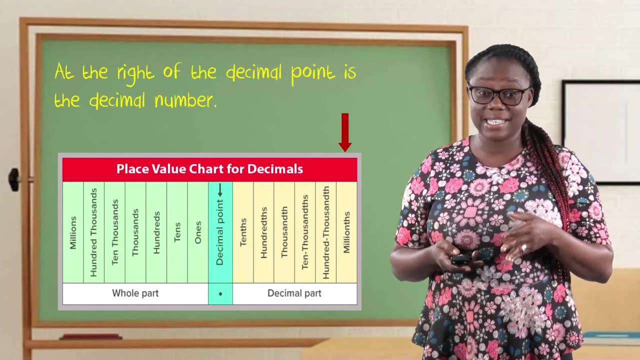 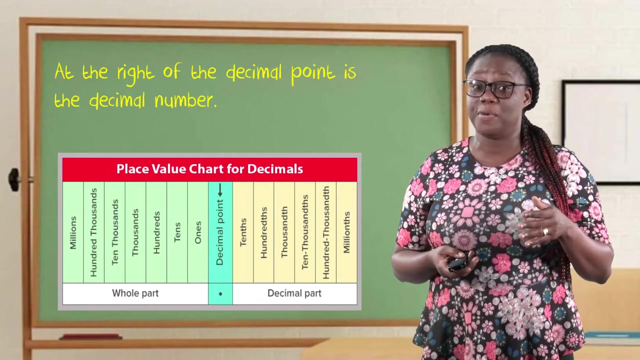 That begins with tenths, hundredths, thousandths, hundredths, hundredths, hundredths, hundredths, ten thousandths, hundred, thousandths and millionths. Boys and girls, are you paying attention? Now, at the right of the decimal point, as we said before, is the decimal number. 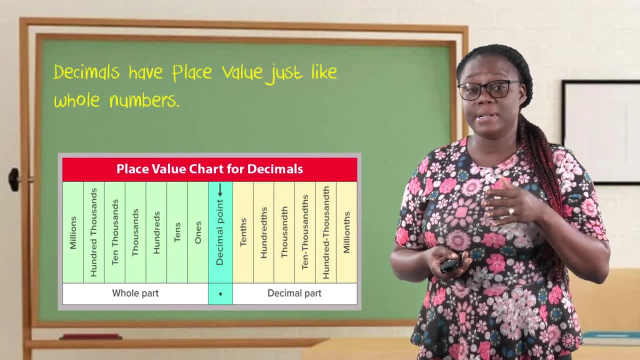 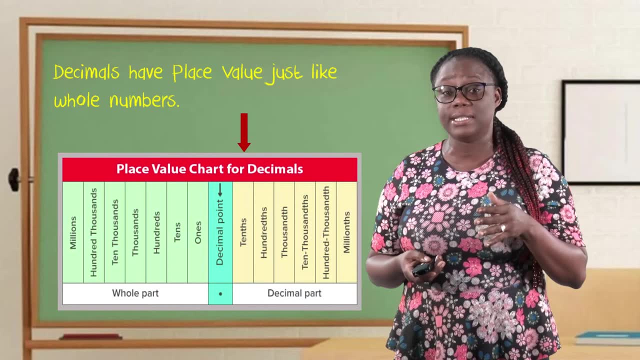 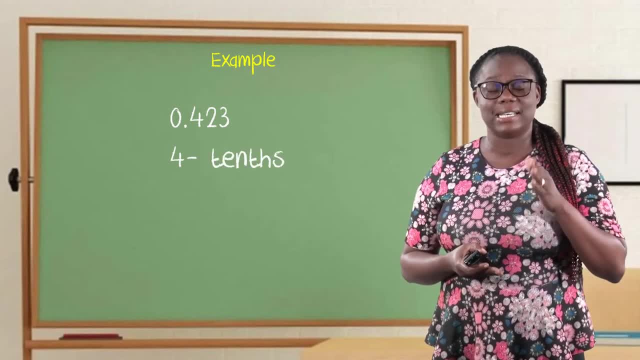 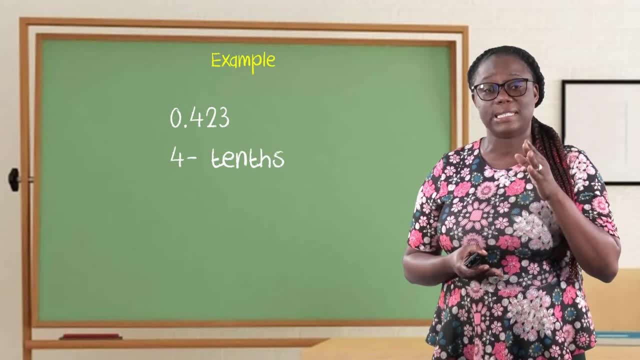 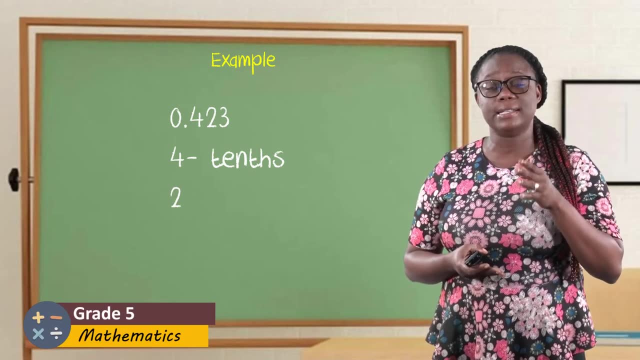 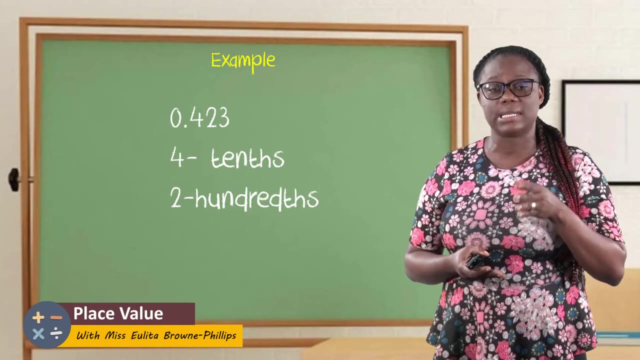 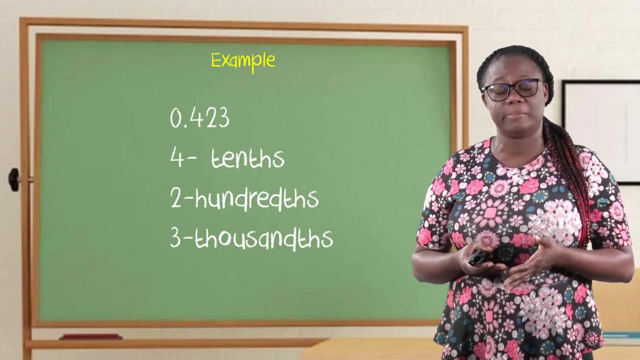 Four falls under the position of tenths. The next number is two. Two is the second digit after the decimal place, And the position that two holds is hundredths. Three is the third digit after the decimal place. Three is positioned under thousandths. 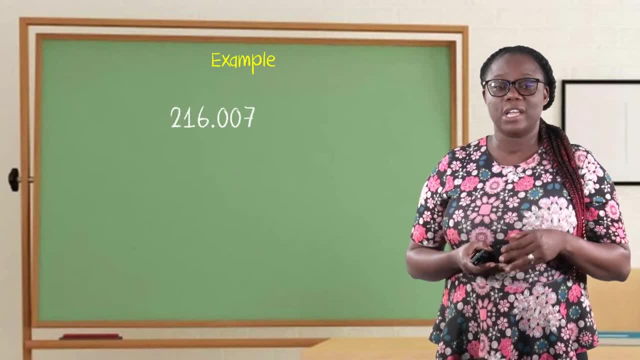 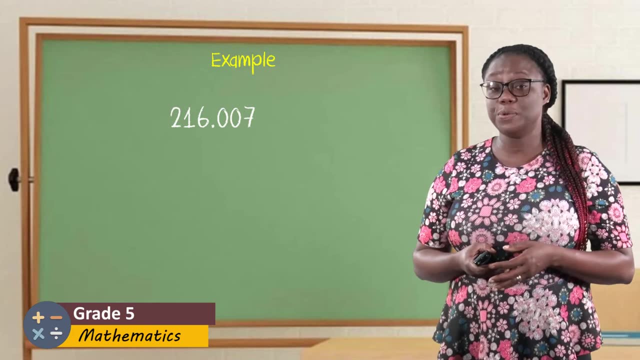 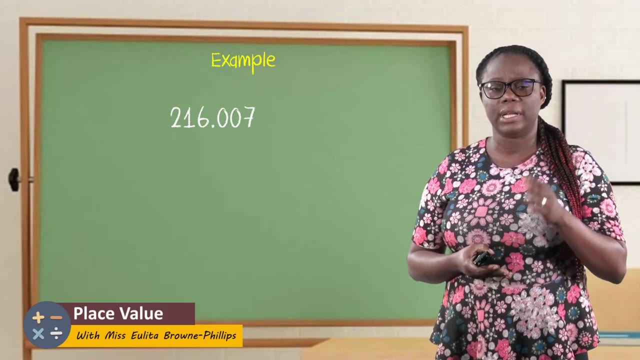 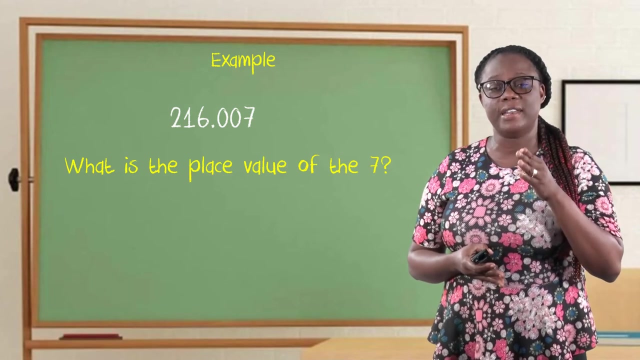 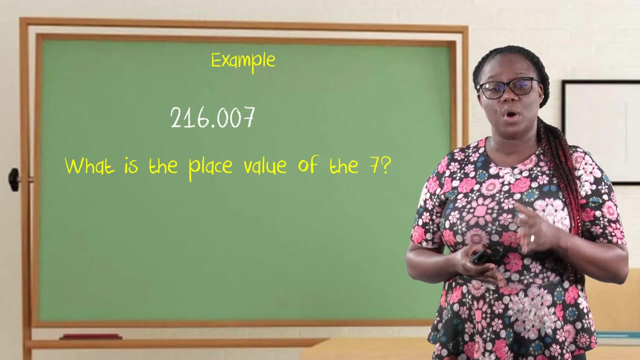 Let's look at another example: 216.007.. 216.007.. Let's look at the decimal part of the number. What position is the seven in? Let's count the number of places after the decimal point: One, two, three. 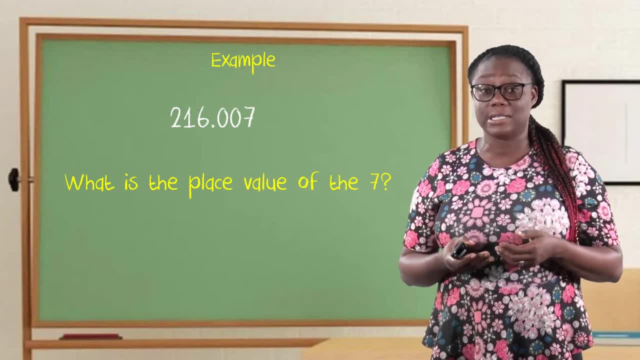 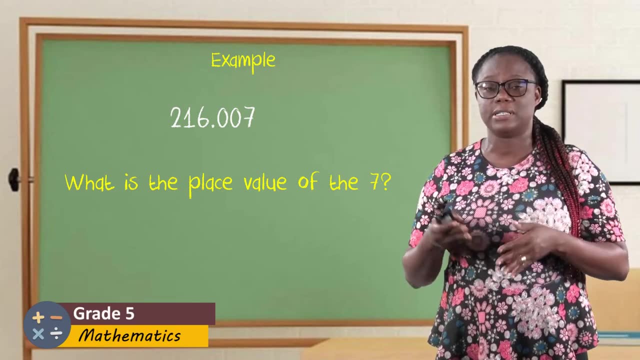 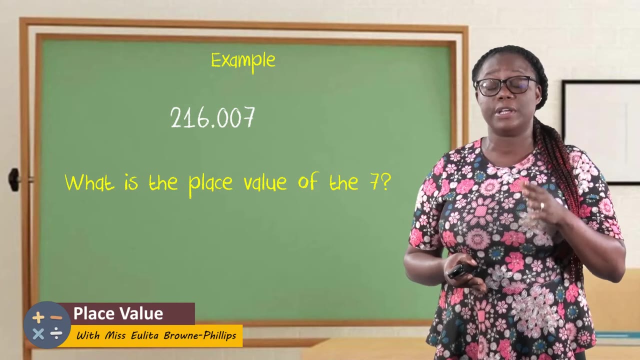 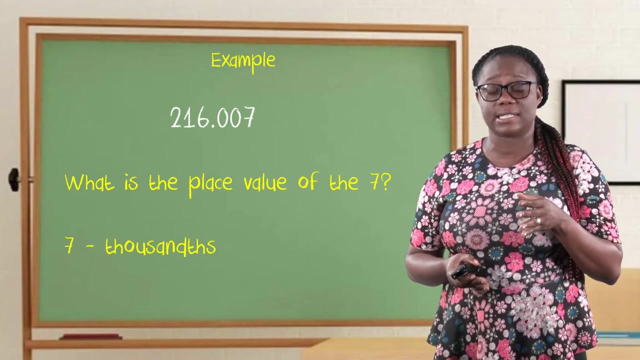 Seven is in the third place after the decimal point. Remember, when we're reading the place value of the decimal, we read from left to right. The third digit after the decimal place is called thousand. So seven is positioned under thousandths. So the place value of the seven in the number 216.007 is thousandths. 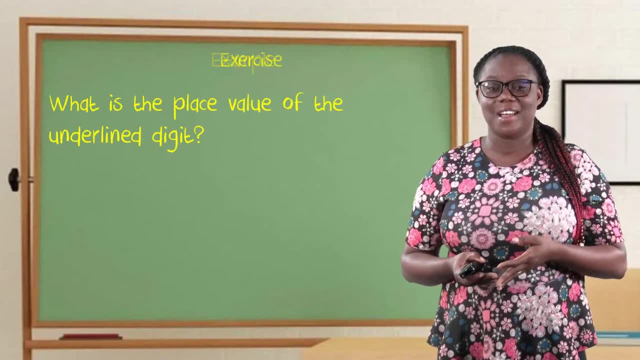 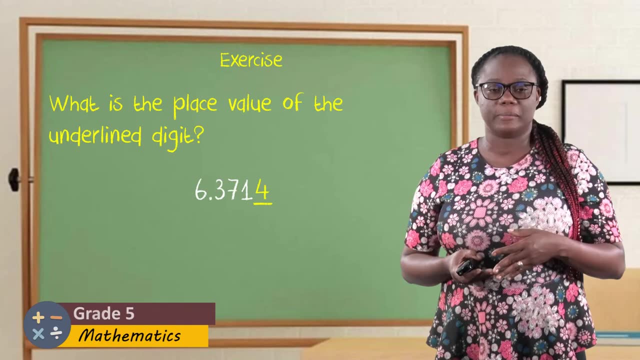 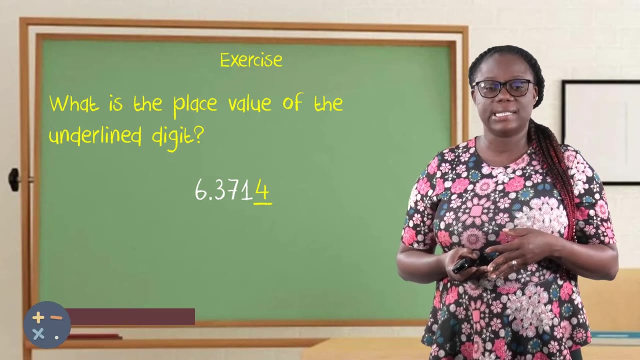 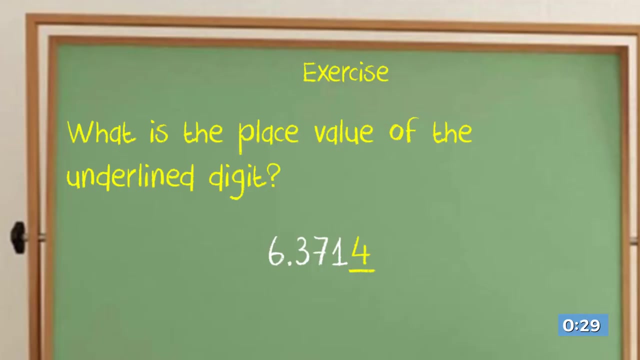 Boys and girls, it is your turn. What is the place value of the underlined digits? The first one, six. The second digit after the decimal point is called thousand. The third digit after the decimal point is called thousand. What is the other arrow? 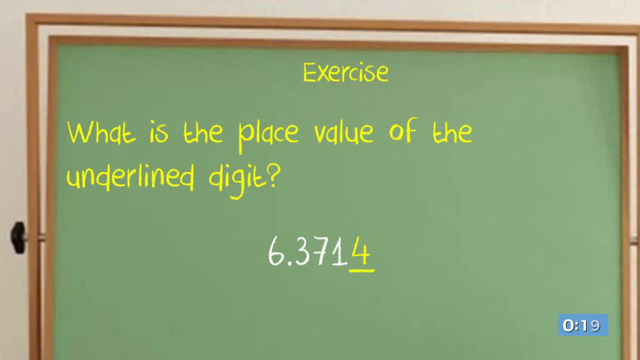 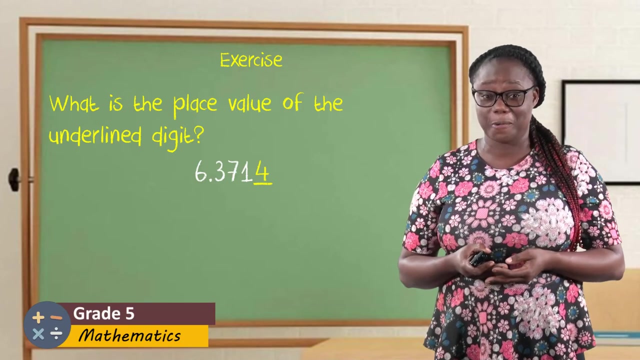 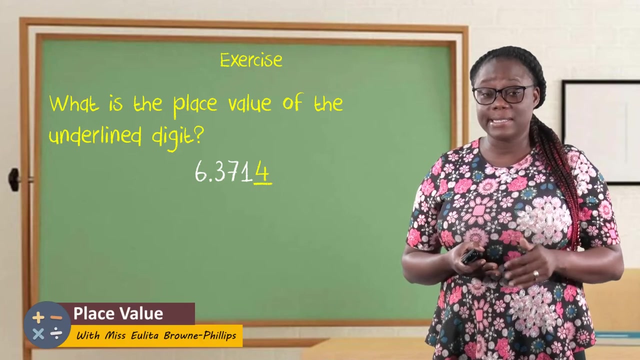 left side, The fourth digit after it. What is the third digit? Eight digit, Nine digit? Okay, you should be finished by now. Let's examine this so that we can have the correct answer. How many places after the decimal point is 4 positioned? 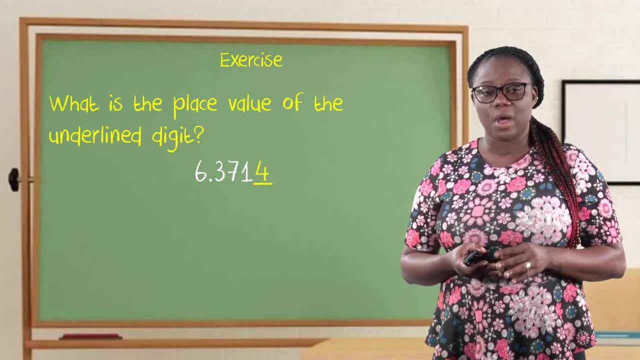 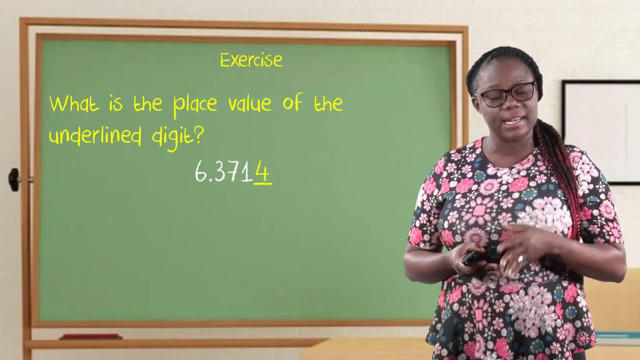 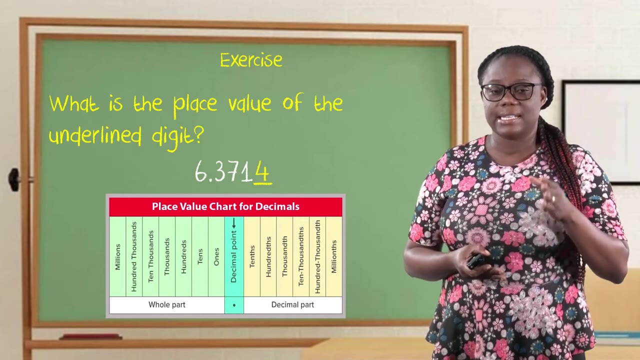 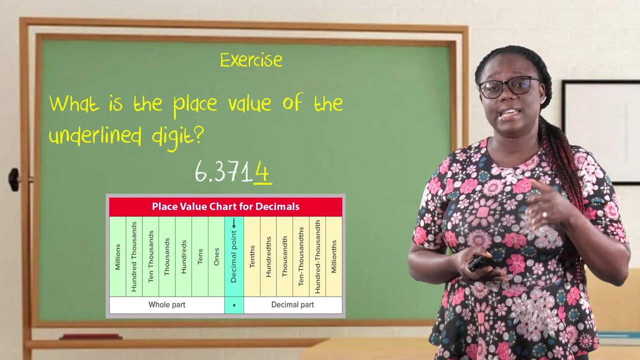 4 places. What do we call the 4th position after the decimal point? Let us go back. The 1st position is tenths. The 2nd position is hundredths. The 3rd position is thousandths. The 4th position is ten thousandths. 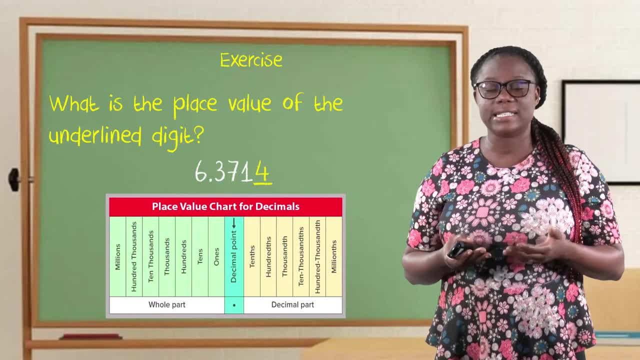 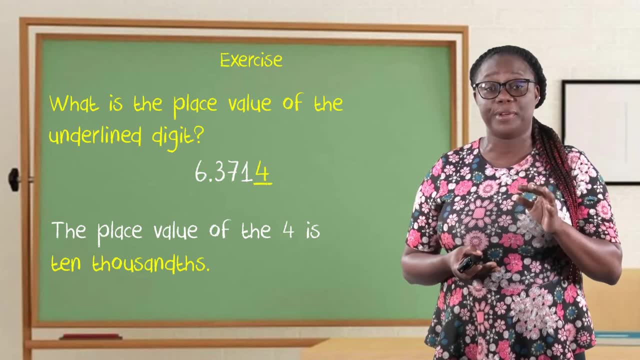 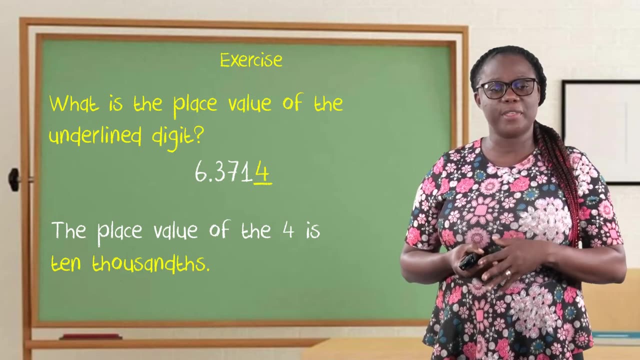 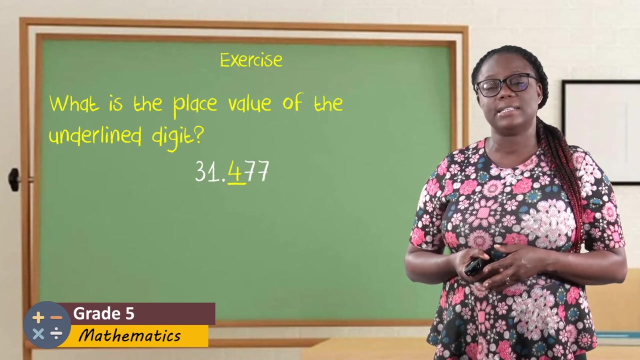 Where is the 4th position Under ten thousandths? So the place value of the 4 in the number 6.3714 is ten thousandths. Let's do another one: boys and girls: 31.477, 31.477. 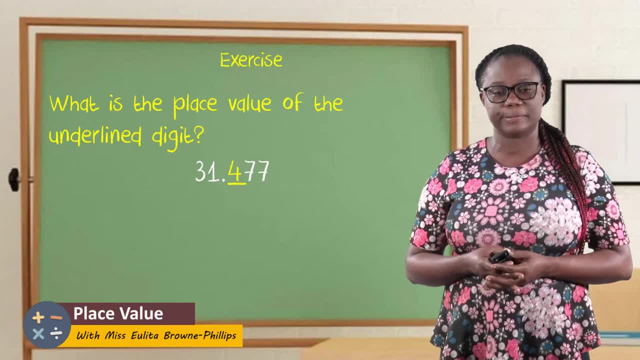 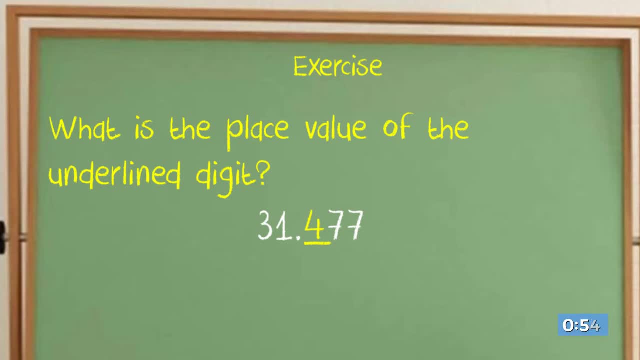 31.477. It takes only one minute to solve the puisse in the paper. The example is 2', which hasprised us and passed out 3. кот 3, 2, 1, 1. 1.. 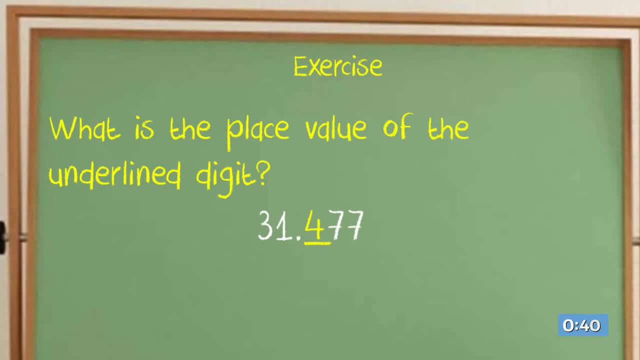 2,看看 2.. 2, подождать. 2, подождать. 3, подождать 4.. 2, подождать 2.. 3: 2 2. 1 2. 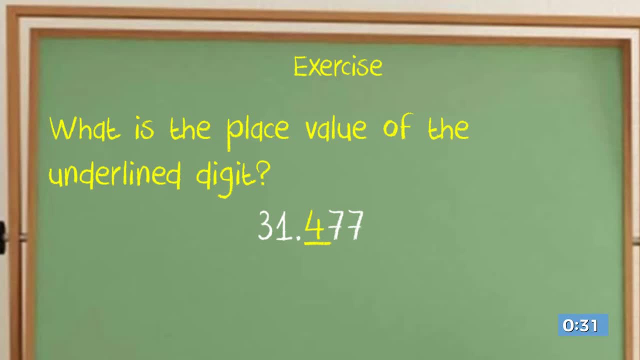 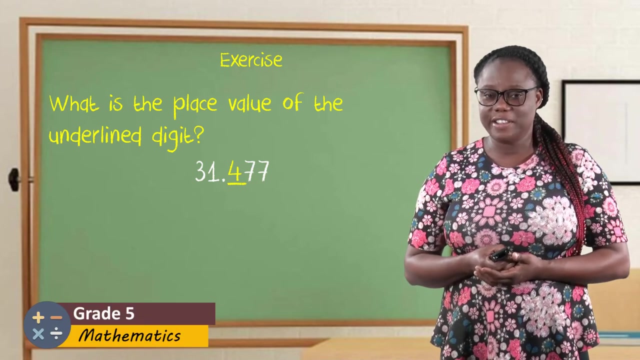 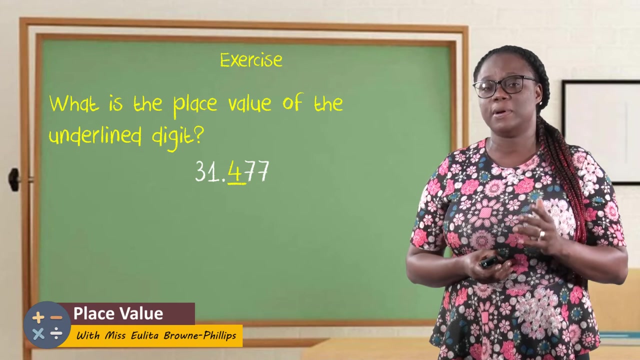 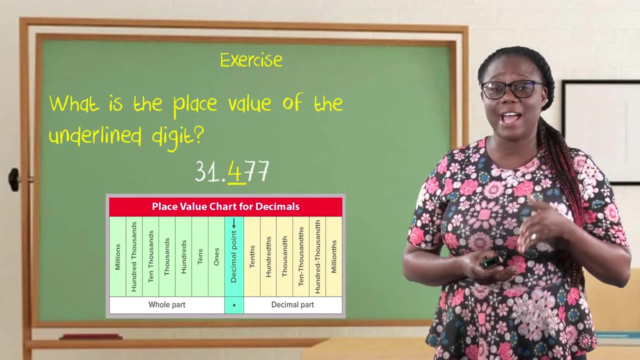 2, 2. Thank you, You should be finished by now. boys and girls, Let's see if we can get our correct answer. How many places after the decimal point is four position? Yes, one place. The place value of the first place after the decimal point is called tenths. 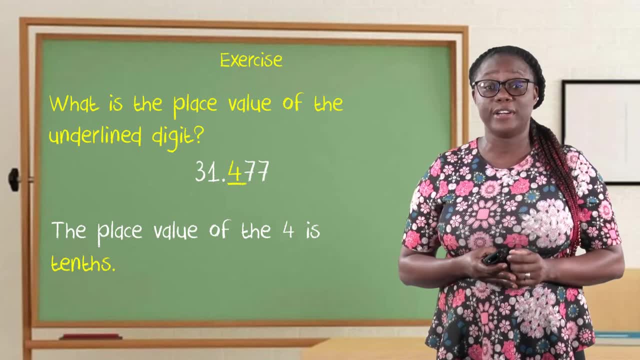 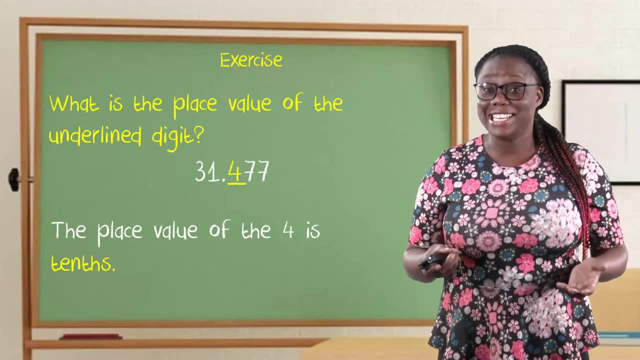 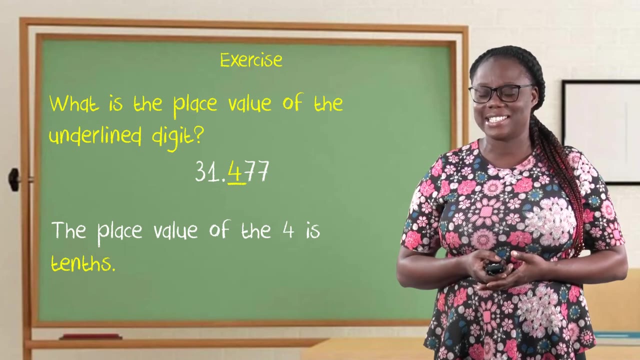 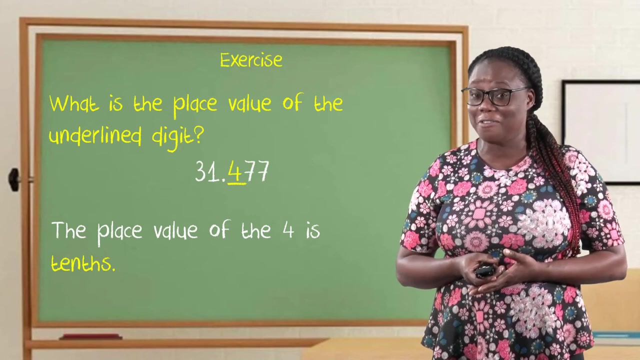 So the place value of the four in 31.477 is tenths. Excellent work, boys and girls. So this has brought us to the end of our lesson, But you know we never close it off unless we have the problem of the day. 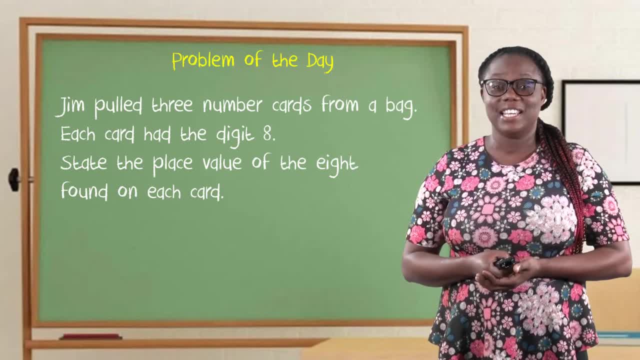 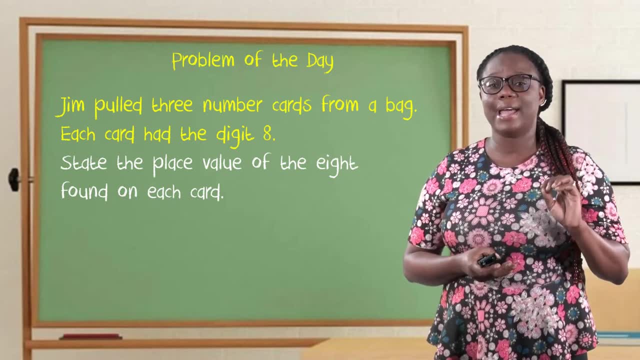 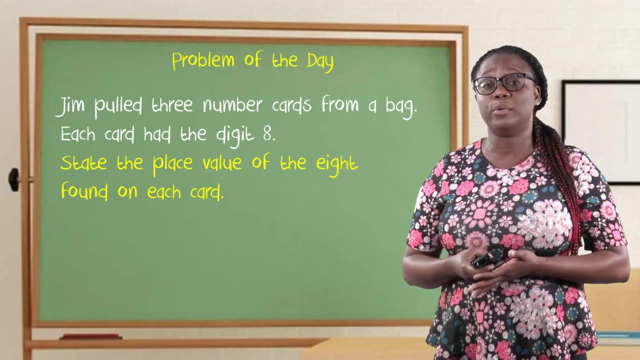 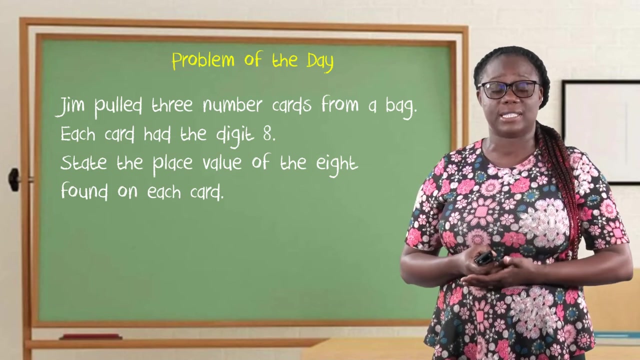 So let's look at the problem of the day, boys and girls. Jim pulled three number cards from a bag. Each card had the digit eight State, the place value of the eight found on each card. So Jim pulled out three cards and there you have it. 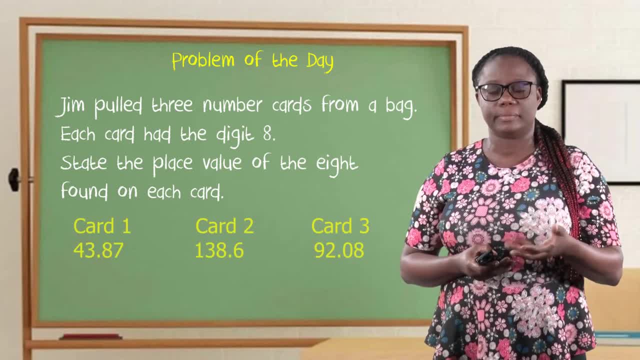 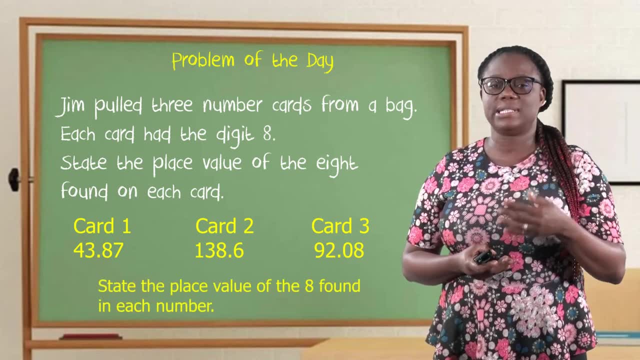 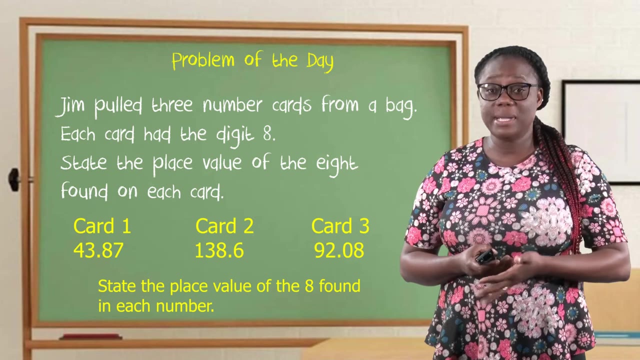 And in each card you have the digit eight. And in each card you have the digit eight, So you will state the place value of the eight found in each number. Take two minutes to do that, boys and girls, And remember to do neat work. 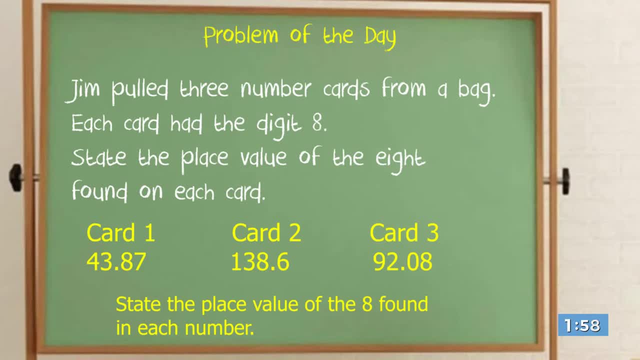 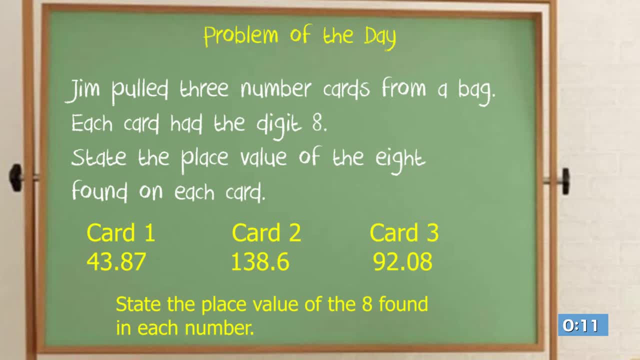 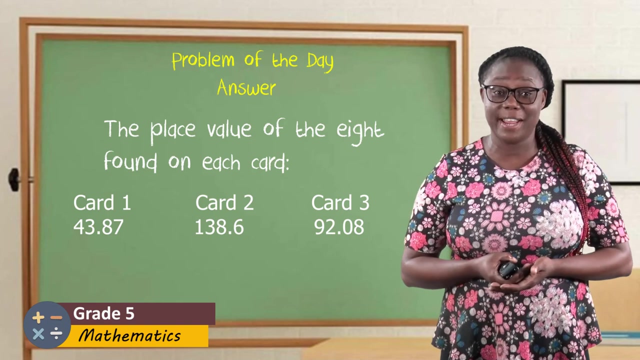 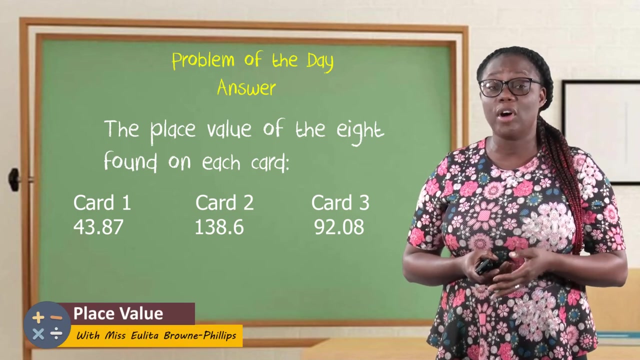 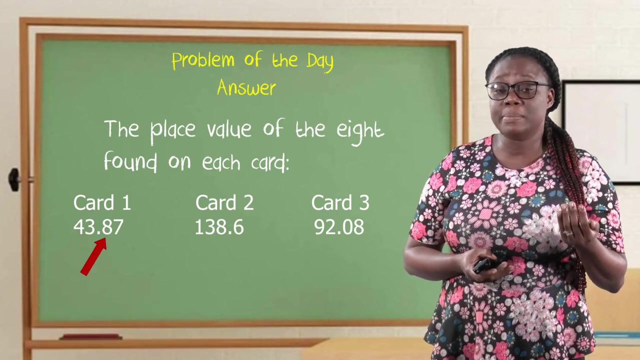 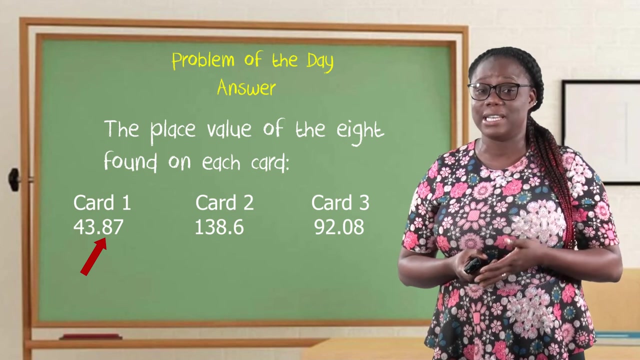 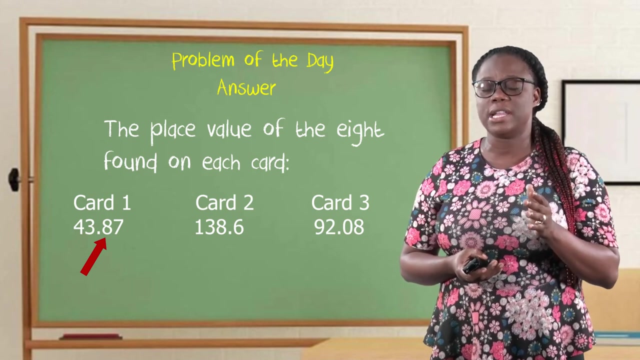 Thank you, Before the decimal point or is it after the decimal point? Yes, it is after the decimal point, So it is a decimal number. What do we call the position after the decimal point? What do we call the first position after the decimal point? 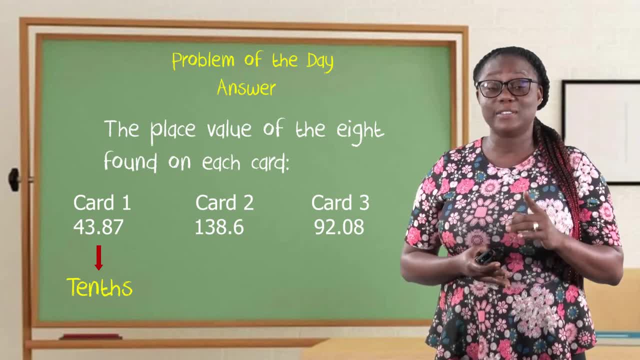 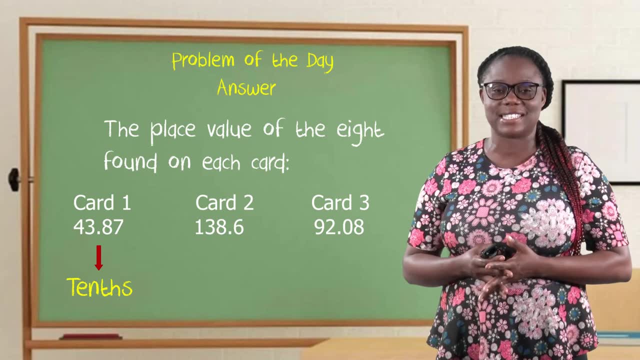 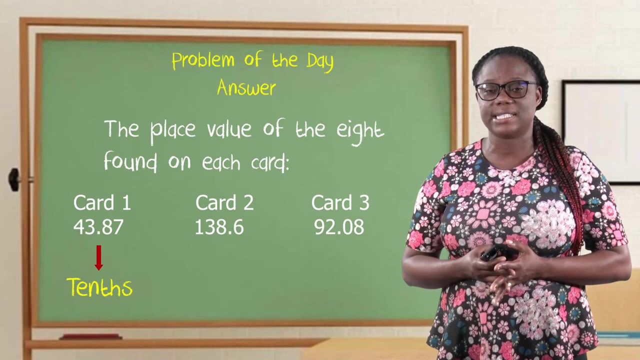 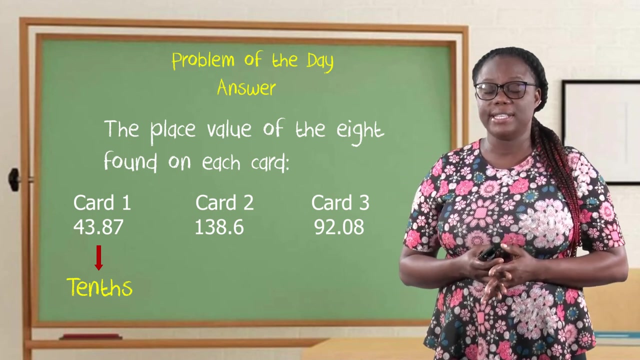 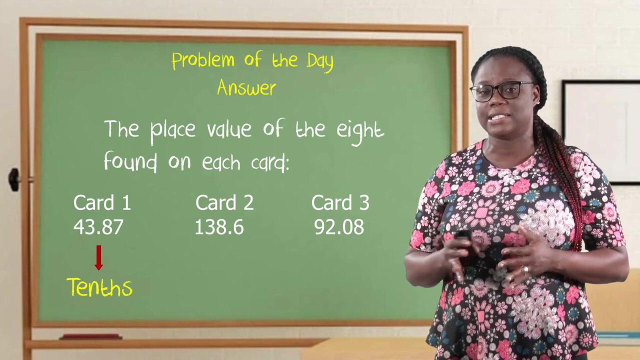 Yes, tenths. So the place value of the 8 and 43.87 is tenths. Let's move on kids. Card number 2, 138.6.. Card number 2, 138.6.. Is the 8 before the decimal point or after the decimal point?